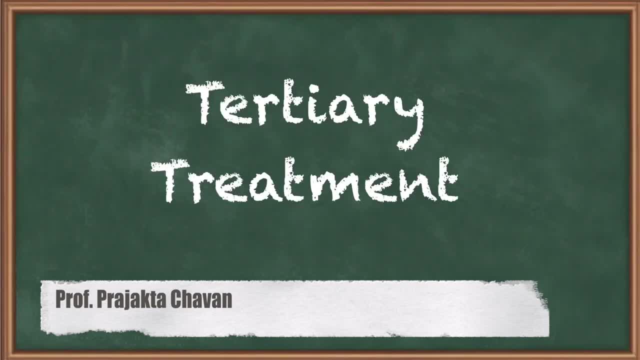 Hello everyone, This is module 4 of the subset of environmental engineering. 2. In previous modules we have already seen the primary and secondary treatments. In primary treatments we have seen the screen chamber and grit removal or grit chamber. In secondary treatment we have seen the different types of treatment like trickling filter, activated sludge process, rotating biological contactors. 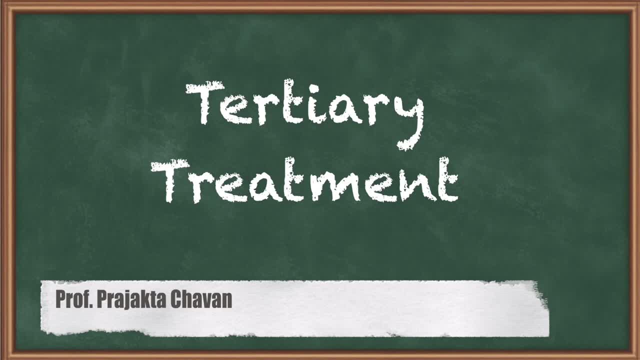 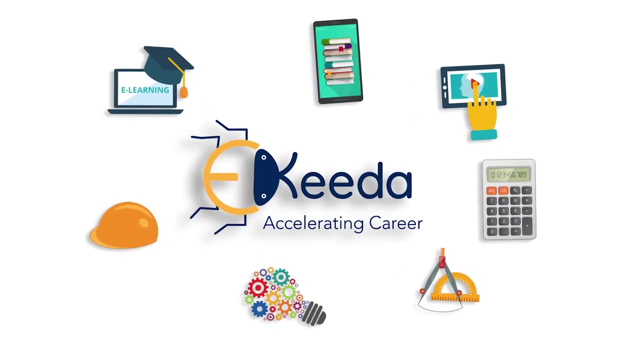 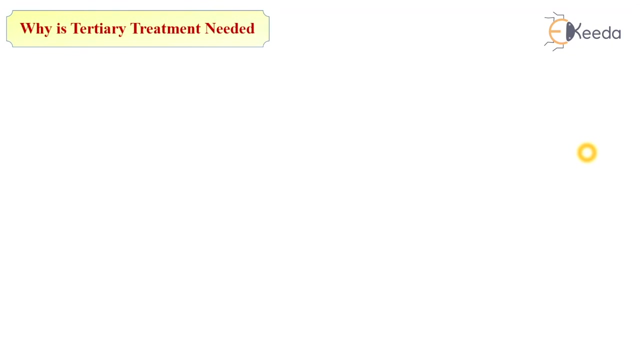 aerated lagoons, wetland, decentralized wastewater treatment systems, etc. So in this module we are going to see the tertiary treatments. What are the tertiary treatments? This treatment is sometimes called the tertiary treatment or advanced treatment and consists in removing the organic load left after the secondary treatment. 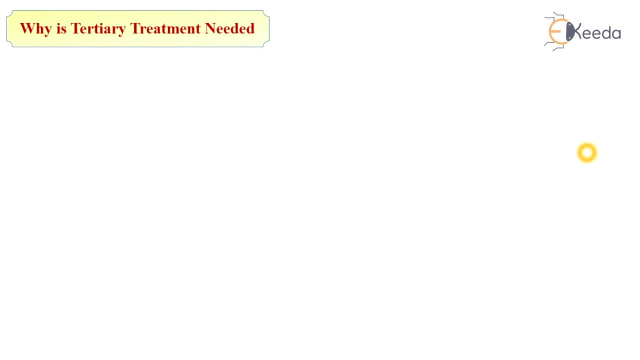 And particularly to kill the pathogenic bacteria. So, as we already discussed on primary and secondary treatment, in secondary treatment we are removing the dissolved particles And in tertiary treatment we are removing the organic matter or very minute size of dissolved particles that we were not removing in secondary treatment. 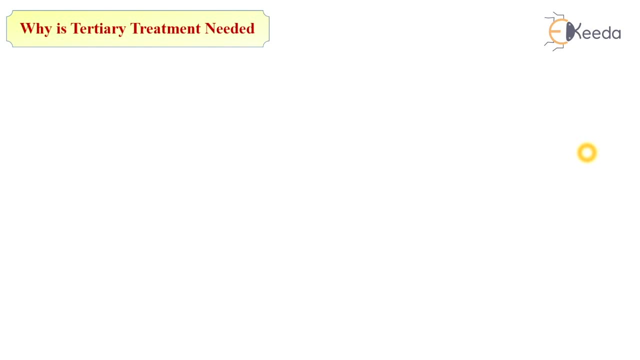 And generally we are removing the pathogenic bacteria in tertiary treatment. So this treatment which is normally So, this treatment which is normally carried out by chlorination, But this chlorination is not carried out for the disposal of sewage in water. 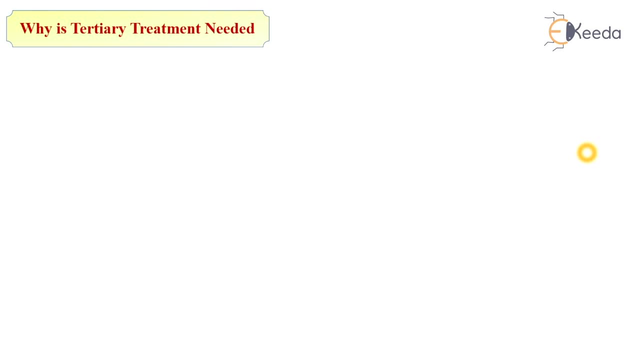 But is carried out while using the river stream for collecting water, for reuse or for water supply. It may, however, sometimes be adopted when the outfall of sewage is very near to the water intake of some nearly town. That means, when the treated sewage is discharged into the water bodies, for example in river and lake, and that water we are further used for the water supply or drinking, then only we are providing the tertiary treatment, chlorination as a tertiary treatment. 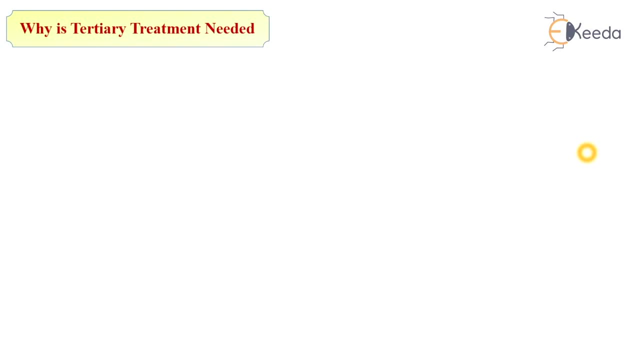 Otherwise for the sewage treatment. we are providing the process till the secondary treatment. So why tertiary treatment is required? To remove total suspended solids and organic matter. those are present in effluent after secondary treatment. To remove specific organic and inorganic constituents from industrial effluent to make it suitable for reuse. 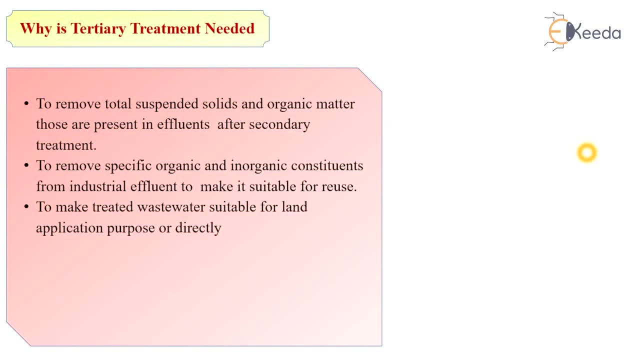 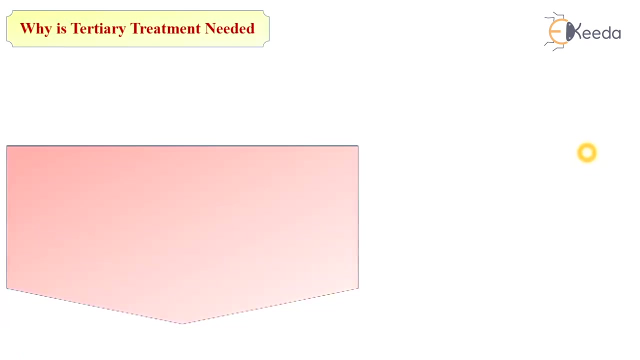 To make treated wastewater suitable for land application purpose or directly Discharge it into the water bodies like river, lake, etc. To remove the residual nutrients beyond what can be accomplished by earlier treatment methods. To remove pathogens from the secondary treated effluent. And to reduce the total dissolved solids from the secondary treated effluent to meet reuse quality standards. 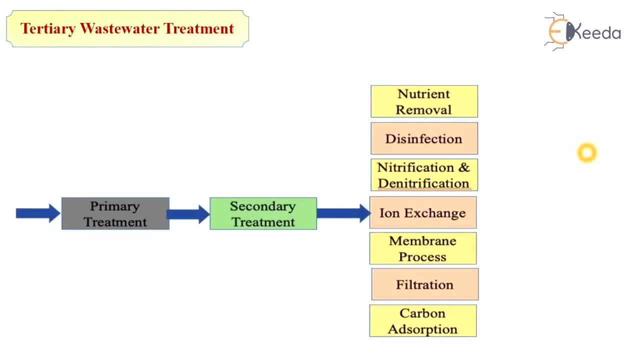 So, as you can see in this video, I am going to show you how to reduce the residual solids from the secondary treated effluent to make it suitable for reuse. So, as you can see in this chart, after providing the secondary treatment, the sewage is go for the advanced treatment or tertiary treatment. 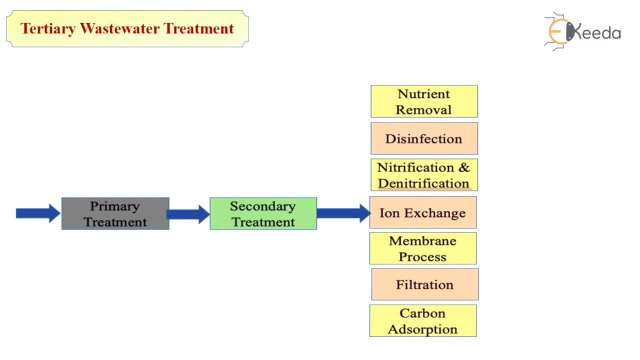 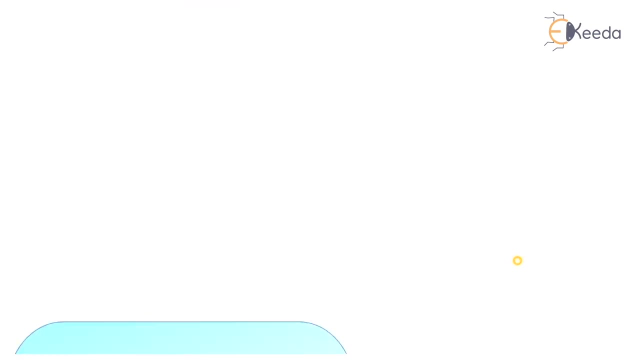 So there are again n number of advanced treatment like nutrients removal, disinfection, nitrification and denitrification, ion exchange, membrane process filtration and carbon adsorption. So let me see one by one. So let me see one by one. 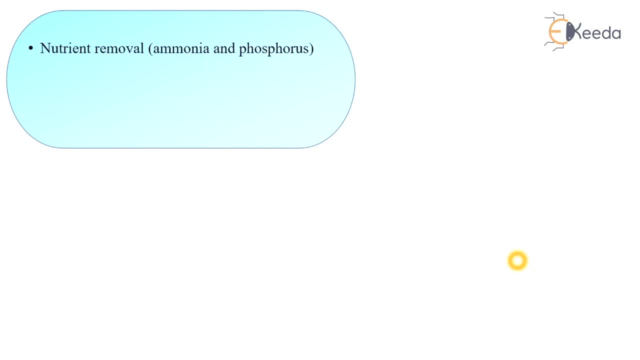 So first is nutrients removal, So first is nutrients removal, So first is nutrients removal. So, after providing secondary treatment, or the effluent is coming from secondary treatment, it consists of nutrients in form of ammonia and phosphorus, And before it will discharge into the water bodies, we are removing them. 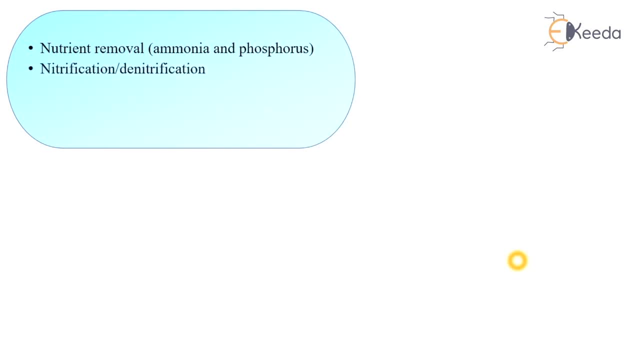 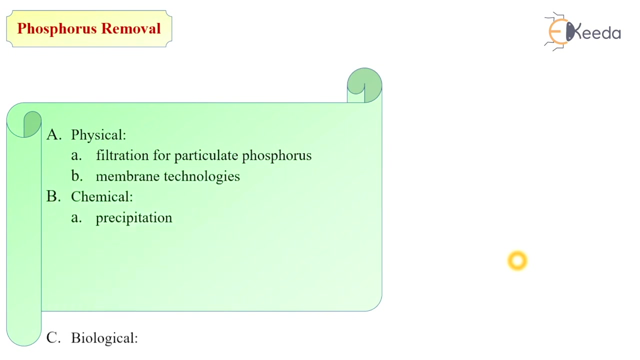 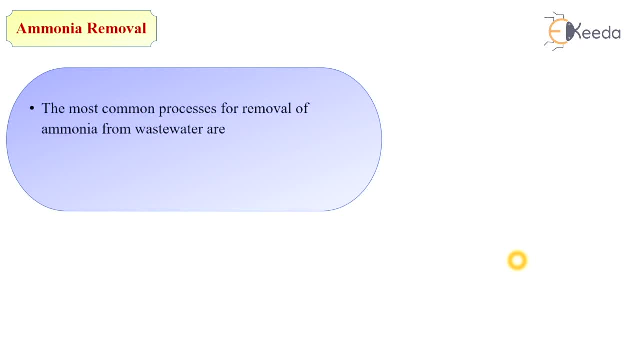 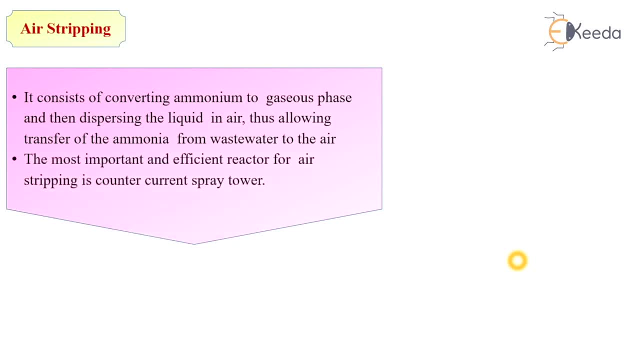 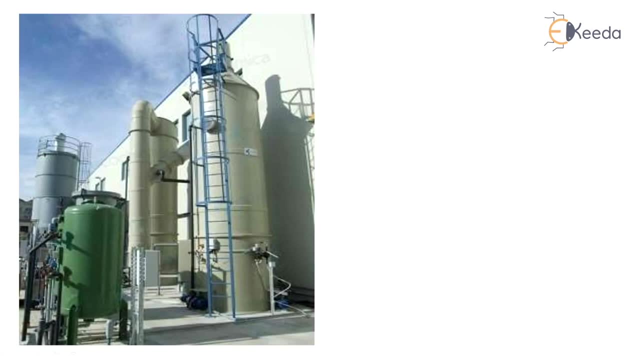 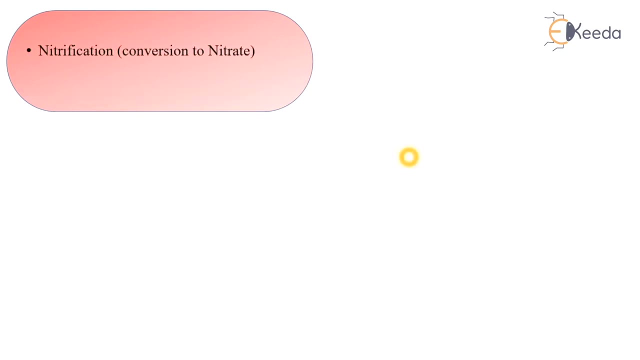 air. The most important and efficient reactor for air stripping is counter current spray tower. So these are the reactor for the air stripping devices. Next is nitrification. Nitrification means conversion of ammonia to the nitrate form And in denitrification. 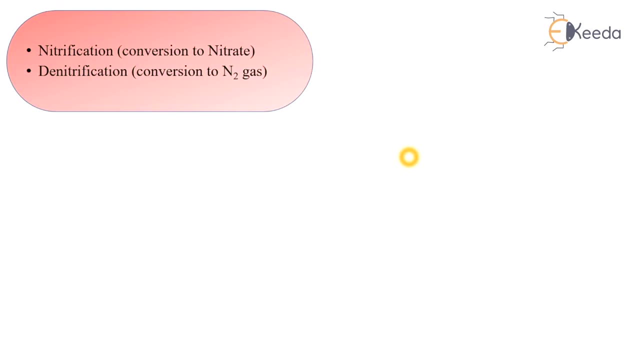 we are again converting this free ammonia or free nitrogen gas to the stable compound. So in denitrification, again we are converting the nitrate to the free ammonia, Then in biological nitrification, the conversion of ammonia to nitrate. So how the conversion is going on. 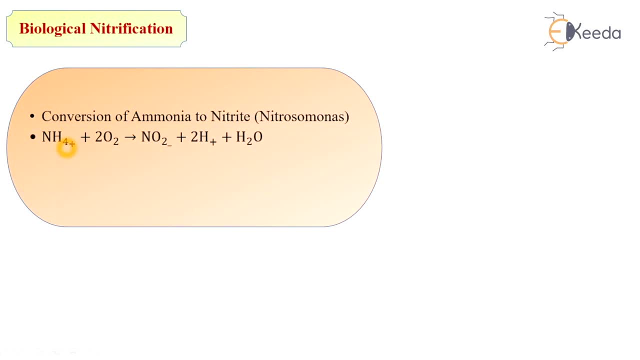 So suppose this ammonia which will get contact in oxygen or air, then this ammonia will convert it into the nitrate. Nitrate is a unstable compound And again this nitrate compound will get oxidized in presence of oxygen and it will get converted to nitrate, that is stable compound. So this 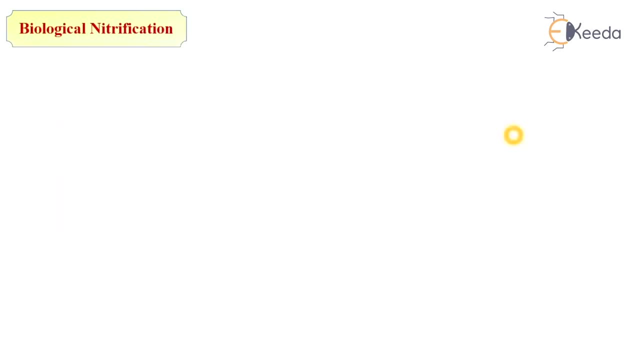 process is called nitrification. So in denitrification the denitrifying bacteria obtain energy from the conversion of NO3, that is, nitrate, to nitrogen gas, but require a carbon source. So for nitrification we are requiring the oxygen to converting this nitrogen gas to the nitrate compound. 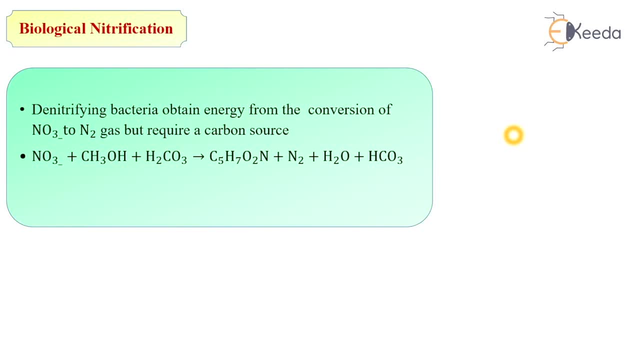 And denitrification is the reverse process. That means we are requiring its conversion from nitrate to nitrogen. nitrogen it will require the carbon source. So, as you can see, in this reaction, this is the nitrate compound and in anaerobic condition, or while the less oxygen will provide, it will. 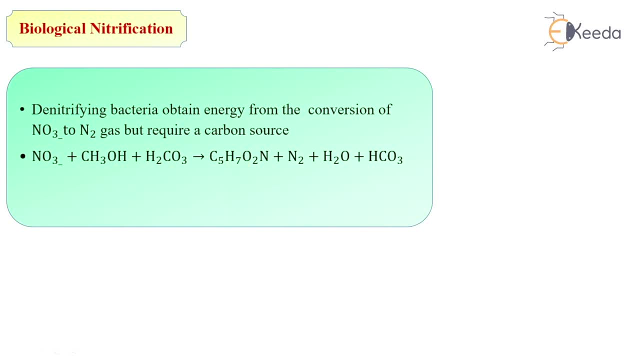 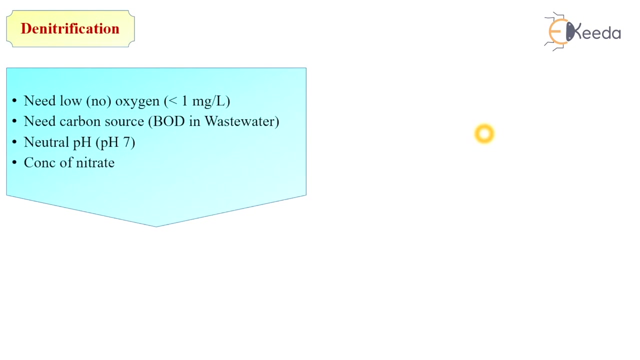 get converted this nitrate compound to the free nitrogen gas. So in denitrification we need the low oxygen that is less than 1 mc per liter. need carbon source- its pH value should be 7 or it should be a neutral- and concentration of nitrate. The next important process we are 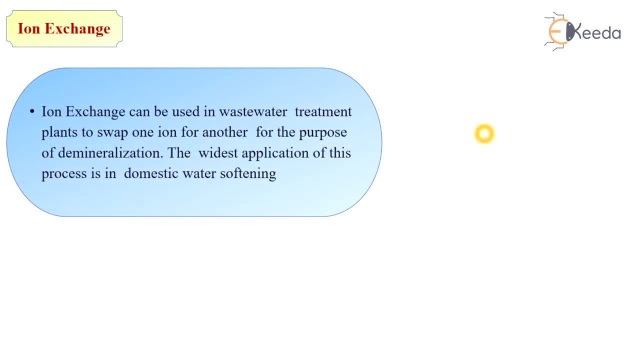 considered as a tertiary treatment is ion exchange process. So in ion exchange. ion exchange can be used in wastewater treatment plant to swap one ion for another for the purpose of demineralization. The widest application of this process is in domestic water. softening Next important process- 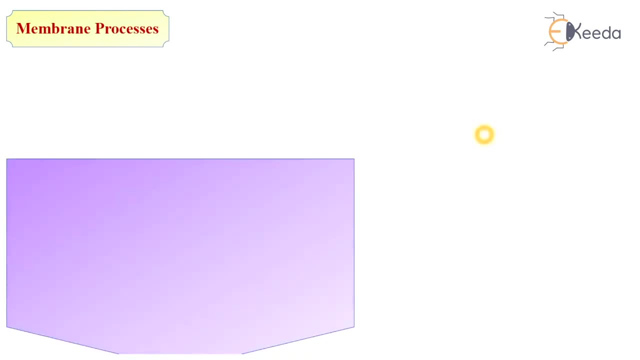 is membrane technology. So there is some classification on membranes. First we will see the what is membrane technology. The membrane process can be classified into sub processes such as micro filtration, ultra filtration, nano filtration and reverse filtration. So, depending on its size of filter media, it will classified as micro, ultra and nano filtration. and 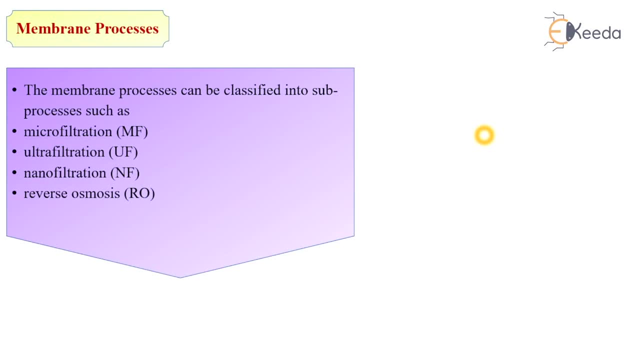 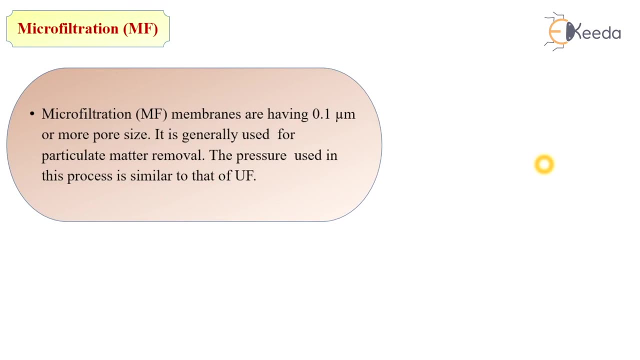 also reverse osmosis in is one of the membrane technology. So let's we will see one by one processes. So first is micro filtration. The micro filtration membranes are having 0.1 micrometer or more pore size. It is generally used for particulate matter removal. The pressure used in this process. 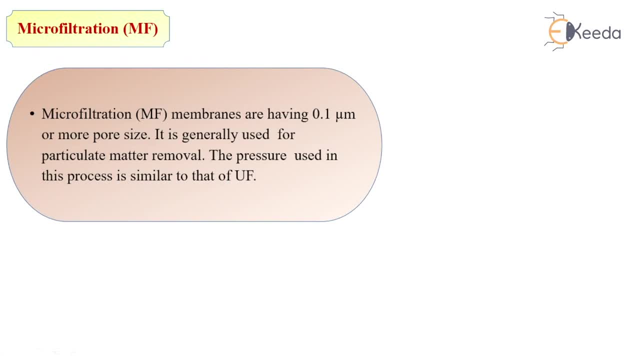 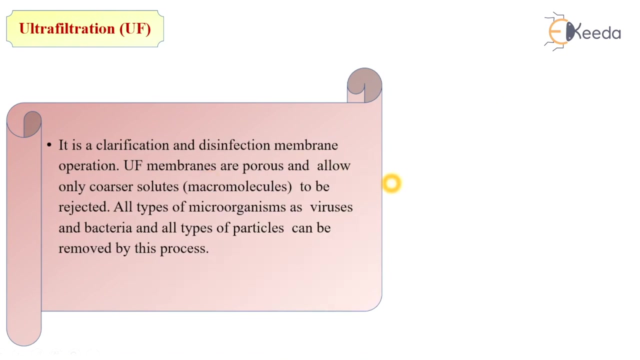 is similar to the ultrafiltration, So the pressure used in this process is similar to the ultrafiltration. So depending on its size- that is 0.1 micrometer- this filtration is called as micro filtration. Then in ultrafiltration it is a clarification and disinfection membrane operation. The ultrafiltration- 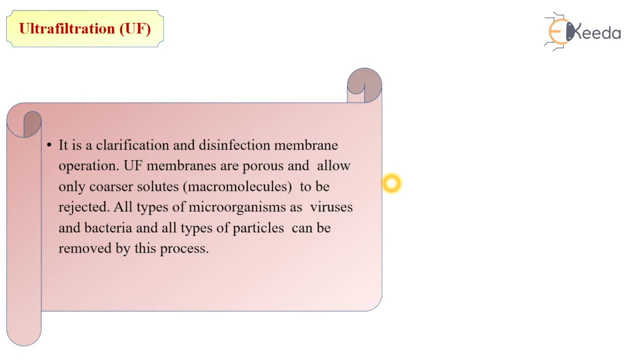 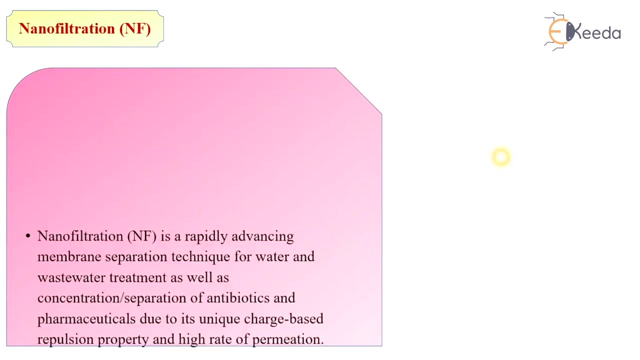 membrane is porous and allows only porous solute to be receipt. All type of microorganism, as viruses and bacteria, and all type of particles can be removed by flocculation The孕 this process, Operating pressure- is kept low as 50 to 500 kPa. In nanofiltration is a rapidly 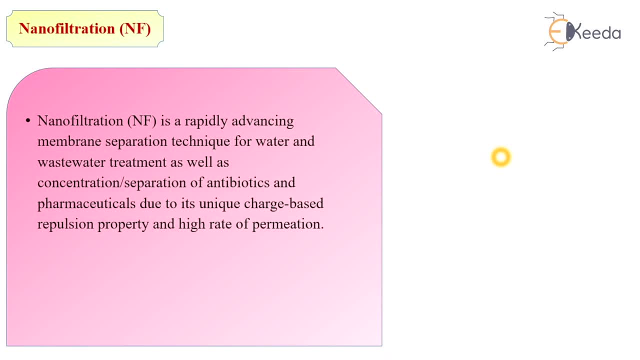 advancing membrane separation technology for water and wastewater treatment, as well as concentration or separation of antibiotics and pharmaceuticals. due to its unique charge-based repulsion property and high rate of permeation, This process is also called as low-pressure reverse osmosis or membrane softening The operating pressure used in nanofiltration. 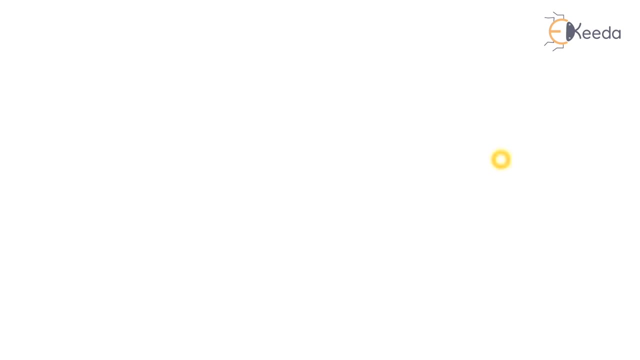 is 0.5 to 1.5 MPa. So next important process is reverse osmosis. Reverse osmosis removes many types of large molecules and ions from effluent by applying the pressure to effluent, which it is an one side of a selective membrane. So reverse osmosis is: 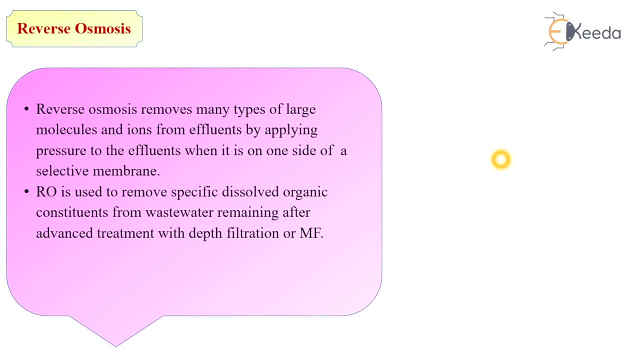 used to remove specific dissolved organic constituents from the wastewater remaining after the advanced treatment. with depth filtration or microfiltration. The reverse osmosis system can operate at 90% of efficiency. Normally, pressure of 5 to 8 MPa is used in this process. 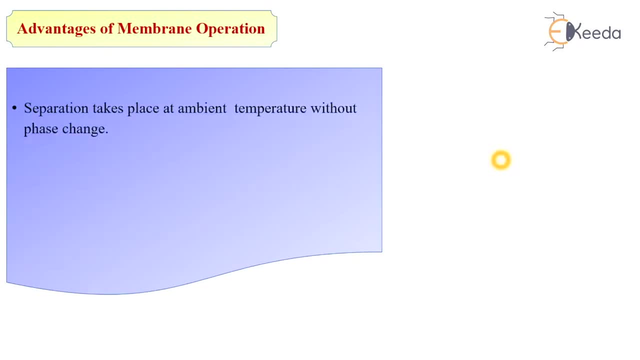 So what are the advantages of membrane technology? Separation takes place at an ambient temperature, without phase change. Separation takes place without accumulation of product inside membrane, unlike ion exchange resins, which needs a replacement or regulations. No need of chemical additives for separation, So it is a physical process. So, according to separation mechanism, membrane. 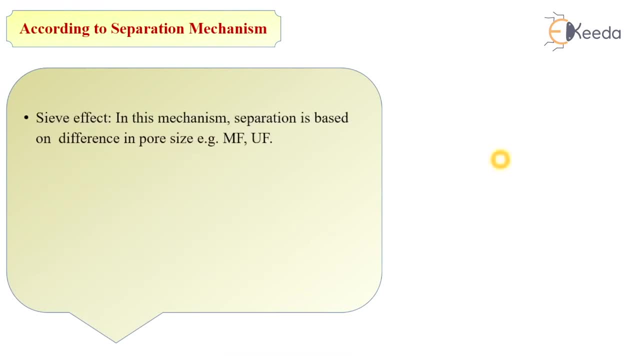 can be separated at an ambient temperature: The sieve effect ie. in this mechanism, the separation is based on difference in pore size. For example, the mechanism happening in microfiltration and ultrafiltration depending on its pore size: Solution diffusion mechanism. In this mechanism, separation is based on difference in the solubility. 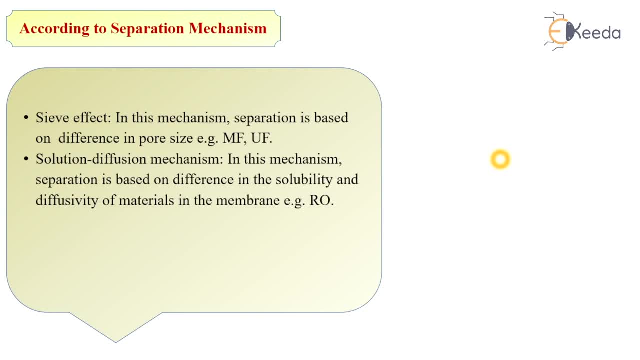 and diffusivity of material in the membrane, which is happening in reverse osmosis, An electrochemical effect, ie. in this mechanism separation is based on difference in charges of species to be separated, ie electrolysis. So microfiltration and ultrafiltration is 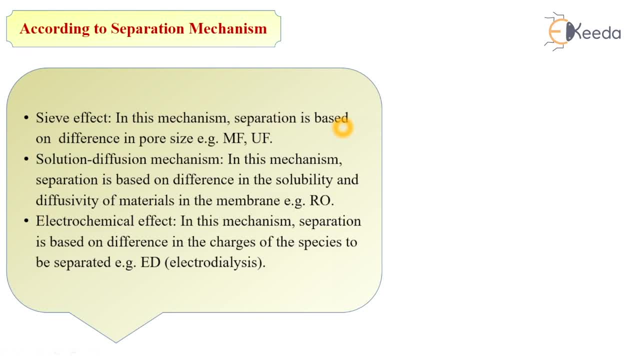 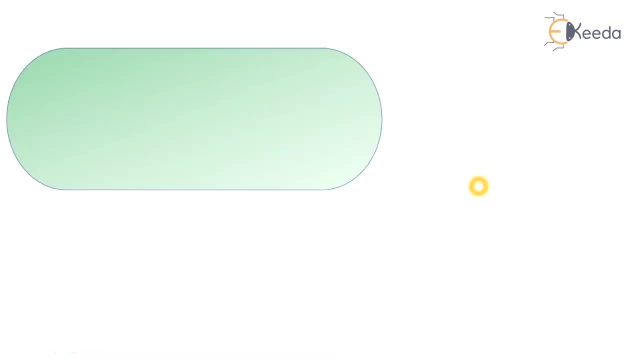 based on sieve effect. ie separation is based on the pore size, The reverse osmosis process is based on the solution diffusion mechanism and electrolysis process is based on the exchange of charges, electronic charges charges. The classification based on separation mechanism leads to two main classes of membranes. 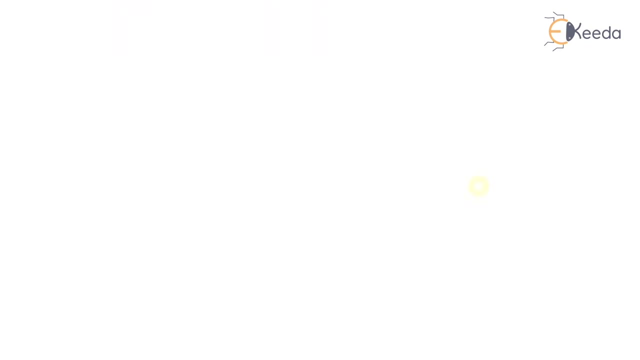 that is, porous membrane and non-porous membrane. So in porous membrane fixed pores are present in this membrane. These pores are subdivided into three types: Micropores. again, it will depend on its size. So micropore sizes is larger than 50 mm. Mesosphere sizes is ranges. 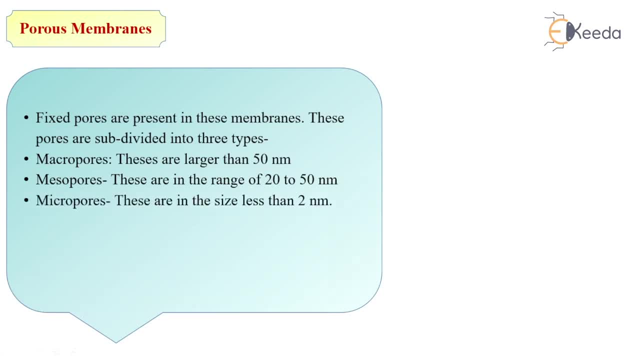 from 20 to 50 mm- sorry, not mm. in nanometer, And for micropores the sizes is vary from or less than 2 nanometer. So microfiltration and ultrafiltration are porous membranes, while nanofiltration could be classified in an intermediate class between porous and non-porous membranes.